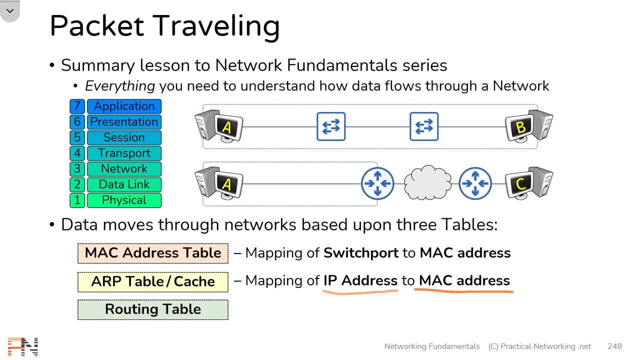 And an ARP table is a mapping of an IP address to a MAC address. A routing table is a mapping of an IP network to an interface or an IP network to an IP address of the next router in the path, also known as the next hop IP address. These three tables are: 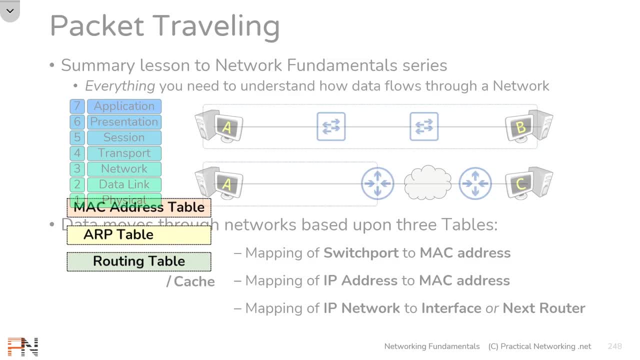 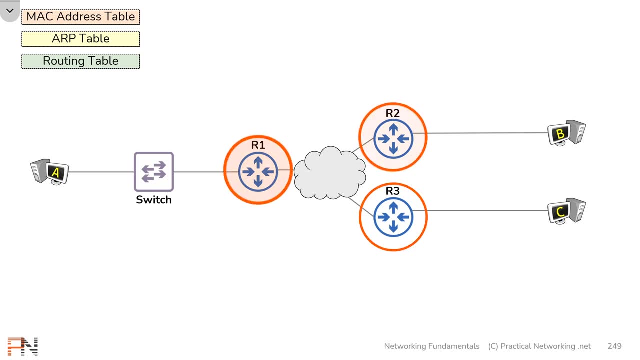 crucial to moving data through a network, And we're going to show you everything that happens with these three tables as data is flowing through this network topology. This topology has three routers- routers 1, 2, and 3, and three hosts: host A, B and C. Each host exists within a network. 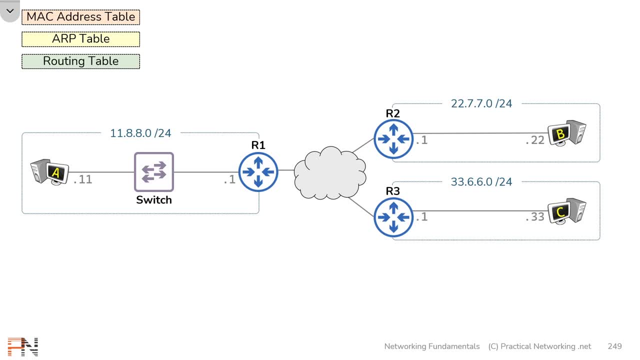 and all the devices have IP addresses in their respective network. And finally, each of these wires are connected to NICs, and each of those NICs have unique MAC addresses. And again, I'm only showing you the first four digits of MAC addresses, to keep things. 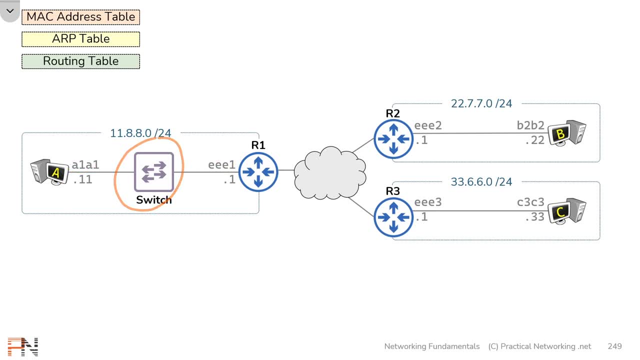 simple Now in the case of the switch. since we're only sending traffic through the switch and not to or from the switch, the switch's MAC address and or IP addresses are irrelevant. We elaborated on this point back in lesson four. So for our switch, 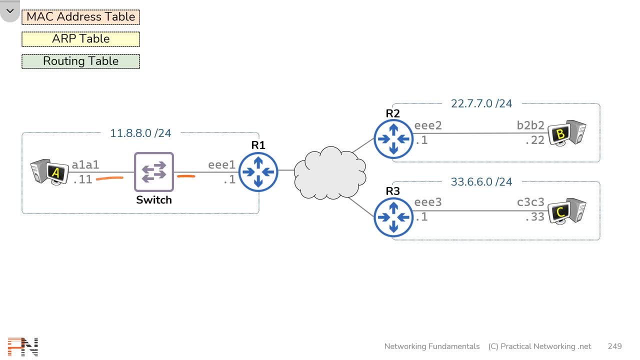 we only need a label for the two switch ports that these wires are connected to. In this case, we're going to be port 4 and port 5.. Each of the devices in this topology are going to use one or more of these tables to process data, And we're going to show them to you in these gray boxes. 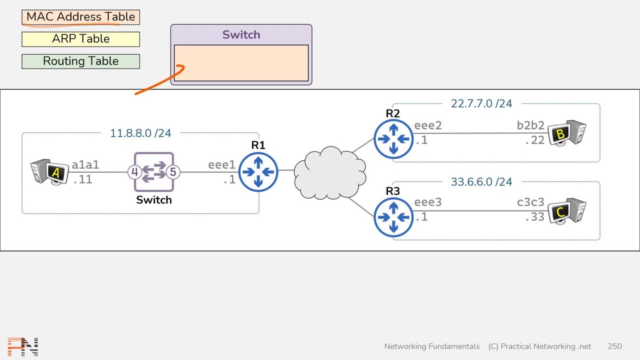 Our switch is only going to have a MAC address table and you're going to see the entries of the MAC address table right there. Our routers have both an ARP table and a routing table, And our hosts being very similar to routers, as we discussed back in lesson five. 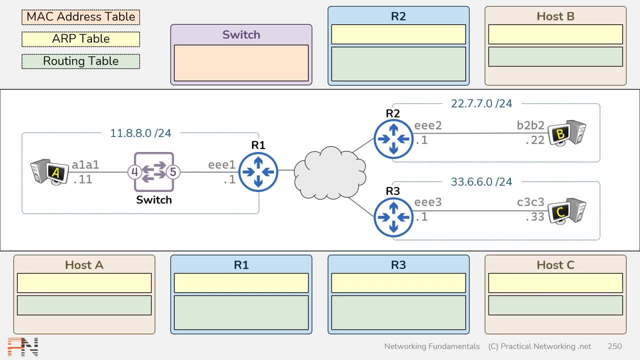 also have both an ARP table and a routing table. The ARP tables are going to be populated dynamically as traffic is flowing through this network. The routing table, however, must be populated ahead of time. Recall that back in lesson five we said that if a router receives a packet with a destination IP address, not in 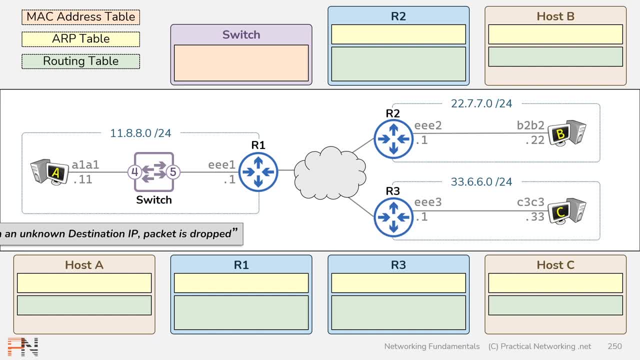 the routing table, that packet would be dropped. So at this point, if our host started sending packets, since our routers have empty routing tables- everything would just be dropped. Therefore, the routing tables must be populated before any data can be sent through this topology. 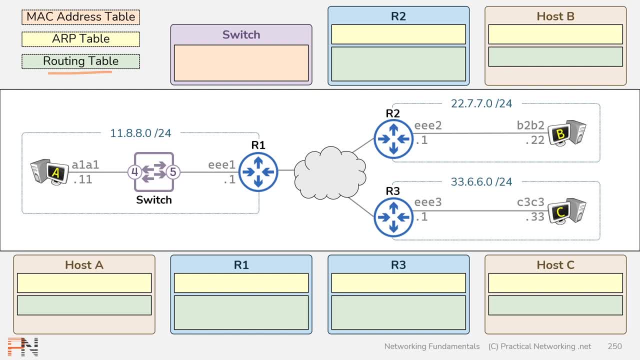 So let's fill in all the entries for all the routing tables in this topology, starting with host A's routing table. Host A only needs a default gateway, also known as a default route. The default route will be represented as a route for the 0.0.0.0. 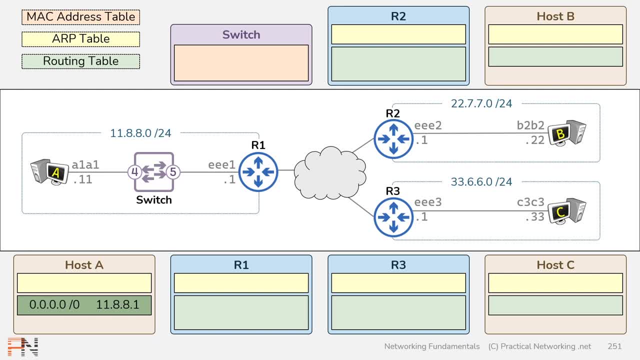 slash 0 network which includes all IPv4 addresses. This route is pointing to the IP address of this interface of router 1, 11.8.8.1.. This will tell host A to use router 1 anytime it's trying to speak to anything on a foreign network. 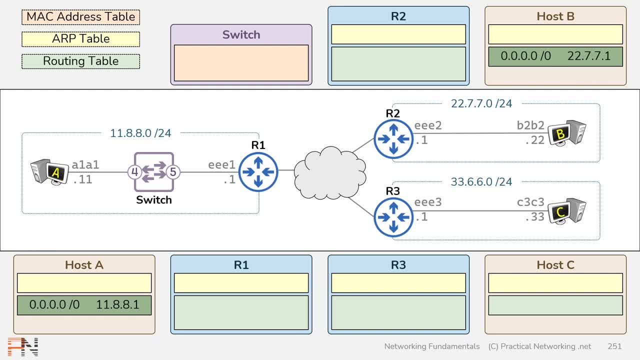 Host B will also have a default gateway pointing to this interface IP address on R2, 22.7.7.1.. And host C will also have a default gateway pointing to this interface IP address on router 3, the IP address 33.6.6.1.. Each of our routers will have two routes. 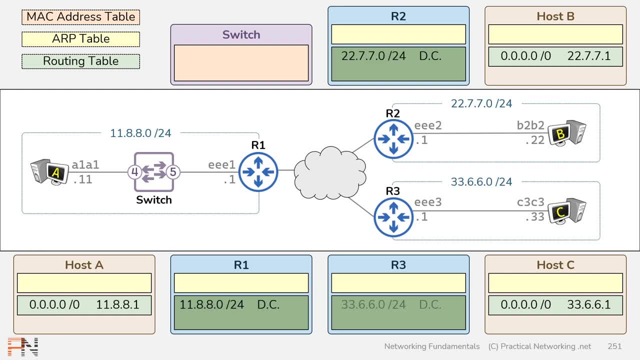 First they will have a directly connected route for the networks that they are attached to. Notice R1 has a directly connected route for the 11.8.8.0.24 network. Then each of the routers are going to have a default route pointing to the internet. 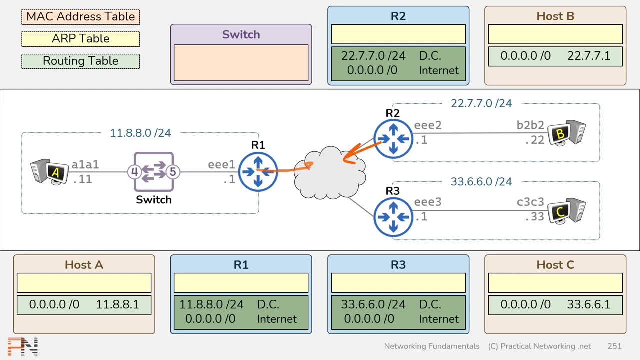 Now, normally that default route would point to a specific router IP address somewhere on the internet. But to keep things simple we'll simply abstract that away and say that this route is pointing simply to the internet. And now we are ready for host A to send some data. 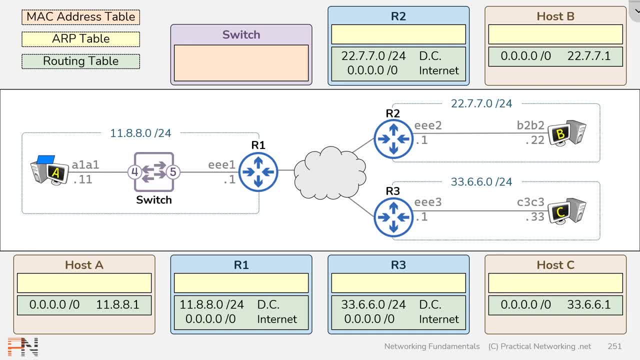 Host A will send the details of this data, but there isn't enough room here to show you the source and destination information. Instead, I'll show you this data in more detail in this box right here. Inside this data payload is just a bunch of ones and zeros. The network doesn't know. 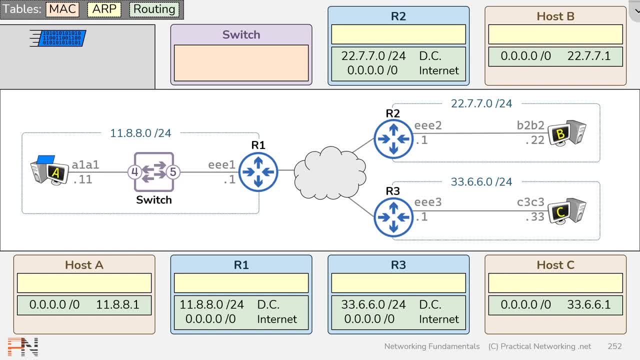 or doesn't care what specifically those ones and zeros are doing. It's just arbitrary computer code that needs to be sent to another host. Host A will start by adding a layer 3 header to this data. This will facilitate the end-to-end delivery of this data. 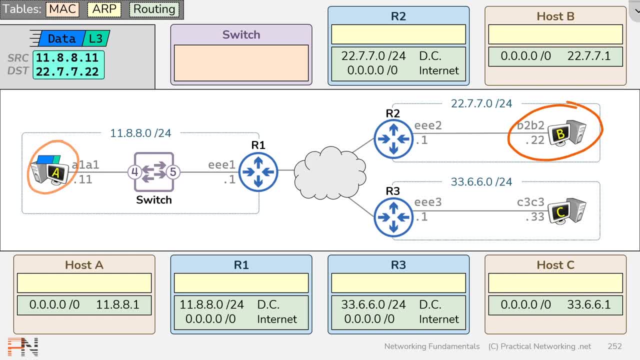 To begin, host A will be sending this packet to host B, So the source IP address of this packet is going to be the IP address of host A, 11.8.8.11.. And the destination IP address of this packet is going to be the IP address of host B, 22.7.7.22.. 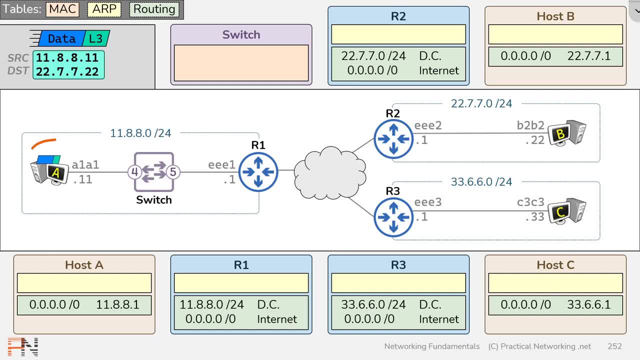 And now we are at the starting point of our illustration and we are ready to follow this packet as it travels through this topology. The first thing that happens when host A is trying to send this data is: host A will compare the destination IP address of the packet with its own IP address and subnet mask to determine that the 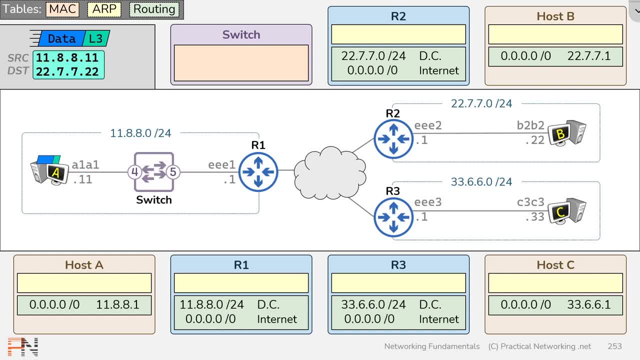 destination IP address is on a foreign network. Therefore, this packet must be sent to host A's default gateway, which is router 1.. But at this point host A's ARP table is empty, which means host A doesn't know router 1's MAC address and therefore is unable to put the. 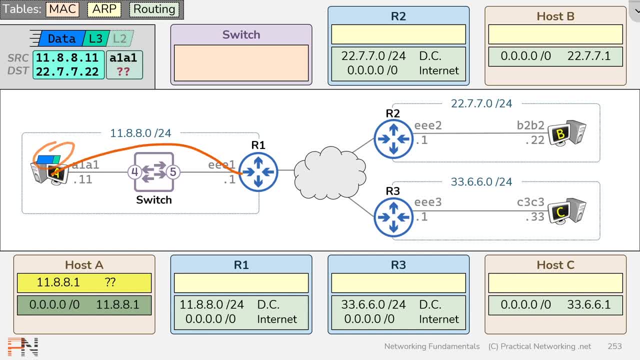 necessary layer 2 header which will take this packet across this hop. So host A will hang on to this packet and first go through the ARP process to resolve router 1's MAC address. The ARP request is also going to have a layer 2 header. That layer 2 header is going to 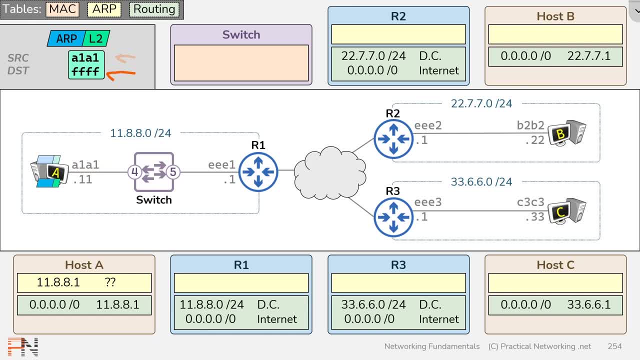 have a source MAC address of host A and a destination MAC address of all Fs. That's the broadcast MAC address. This will tell the network that this ARP request should be sent to everybody in this network. When host A puts that on the wire it'll arrive on our switch. 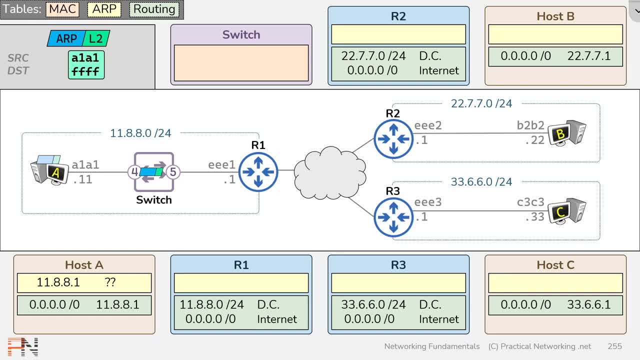 Anytime something is received on a switch, it's going to try and learn the mapping between the receiving switch port and the source MAC address. In this case, the source MAC address of this frame is A1, A1, and the receiving switchport is port 4.. Therefore, our switch is going to. 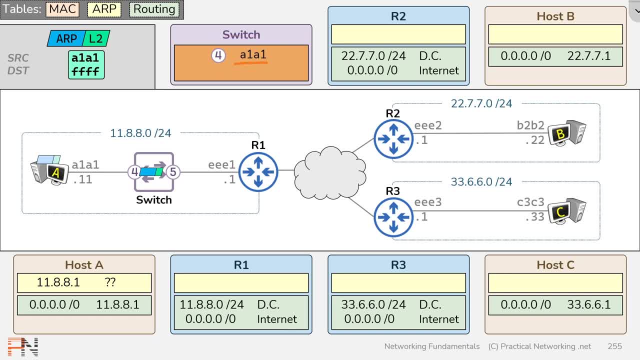 learn that something out port 4 owns the MAC address A1, A1.. Then the switch is going to look at the destination MAC address. In this case, the destination MAC address will be A1, A1, A1, and A2.. The destination MAC address will also look at the AD-enen diferentes MAC addresses, In this case, the destination MAC. 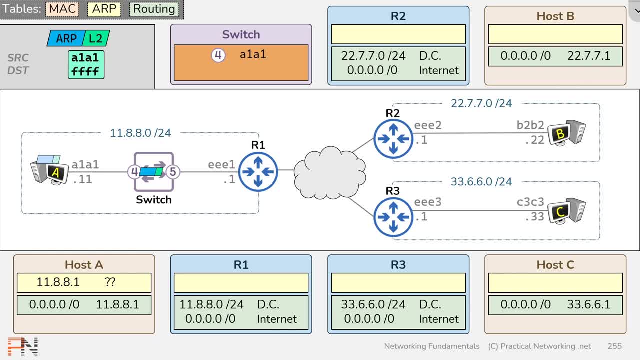 MAC address is all Fs, which tells the switch that no matter what it's going to do the flooding action to send this frame out all ports. Now in our topology there's only two devices in this network, But if there were other devices plugged to this switch they would also receive a copy. 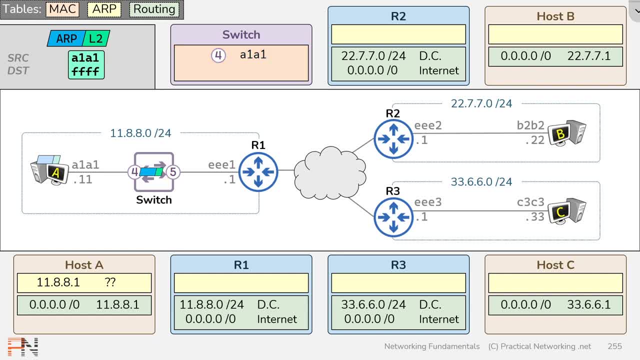 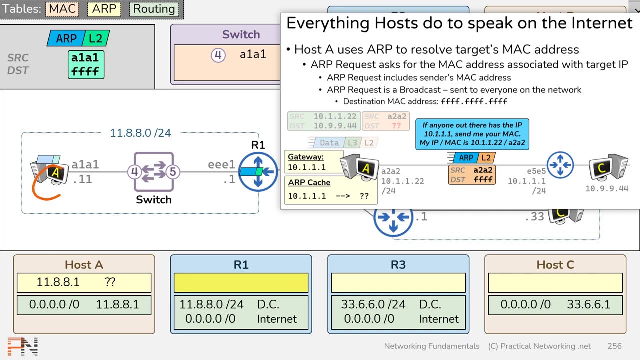 of this frame. But for us that frame would only be sent out port 5, where it'll arrive on router 1.. Upon arriving to router 1, router 1 will get to learn the ARP mapping of the sender. Recall that. when we discussed ARP, we told you that inside the ARP request is the ARP mapping. 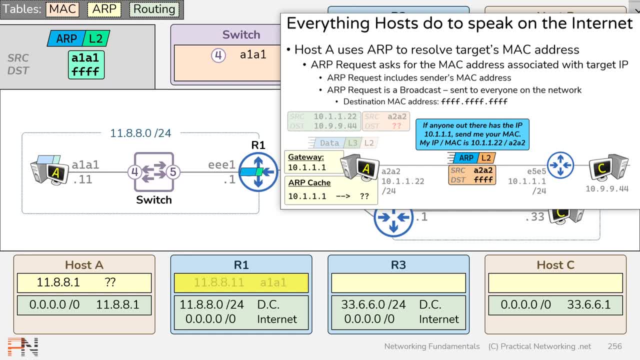 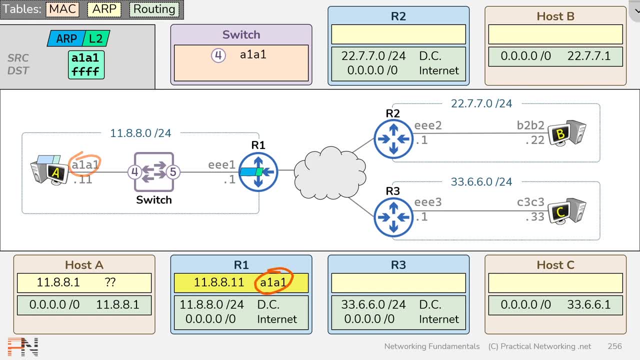 of the sender. So by simply receiving the ARP request, router 1 is able to learn that a device with the IP address 11.8.8.11 maps to the MAC address A1A1.. Then router 1 will generate an ARP. 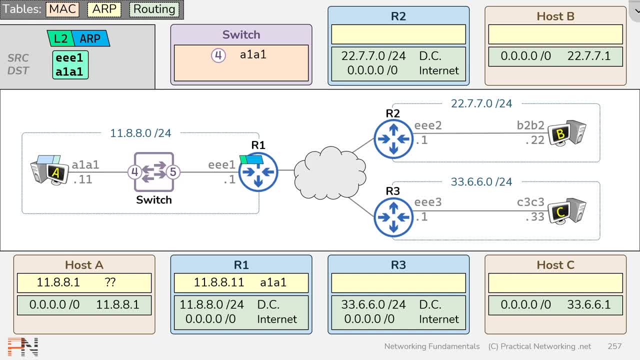 response. This ARP response is going to look like this: It's going to have a source MAC address of router 1's nick and a destination MAC address of host A. The ARP response is going to look like this: It's going to have a source MAC address of host A. 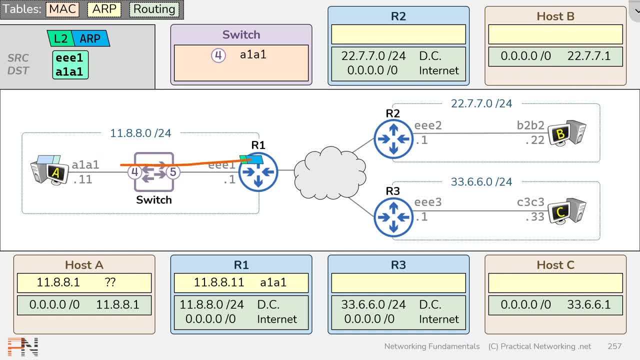 This is a unicast ARP response meant to be delivered directly back to host. A Router 1 will put that on the wire, where it'll arrive on our switch And again, just like before, since the switch received something on port 5, it's able to learn that a device out port 5. 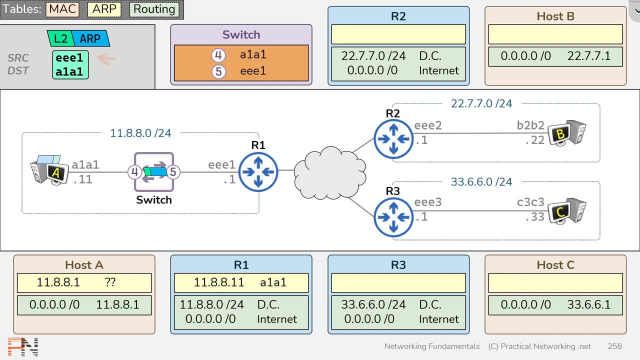 owns the MAC address EEE1.. Then the switch will again take a look at the destination MAC address. In this case the destination MAC address is A1A1, and our switch already knows that that MAC address exists out port 4, and will therefore forward this frame out port 4, where it'll finally arrive. 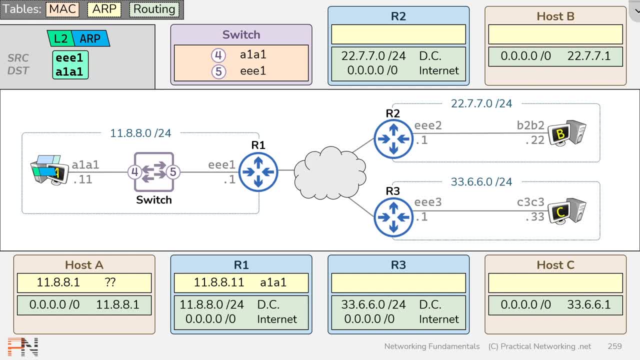 back to host A. Once host A receives it, host A will learn the MAC address that it was trying to resolve, In this case that the IP address 11.8.8.1 maps to the MAC address EEE1.. And now, 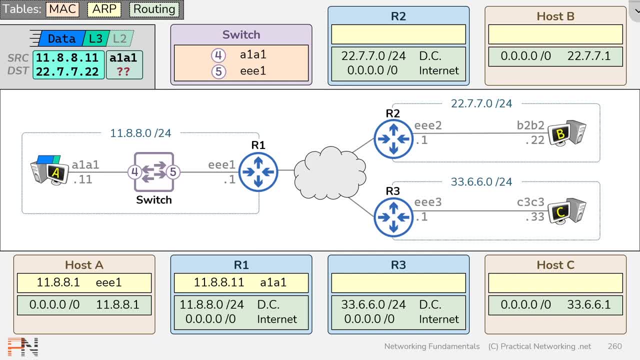 host A has the necessary information to complete this layer 2 header which will take our data packet to the router. That layer 2 header will have a host A address and the host A address will have a have a source MAC address of host A and a destination MAC. 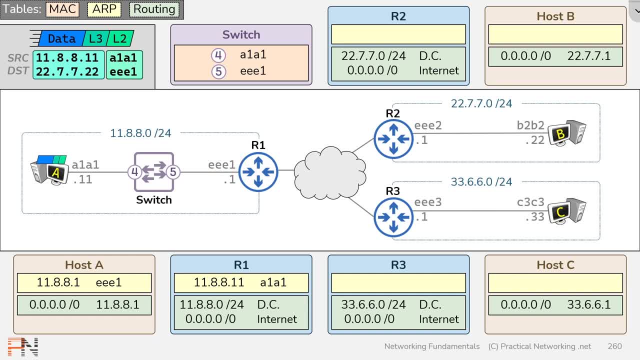 address of the router. now that host A knows the router's MAC address, This Layer 2 header will handle delivering this packet across its first hop, which, in fact, is the goal of Layer 2, hop-to-hop delivery. Now, if that idea isn't familiar to you, 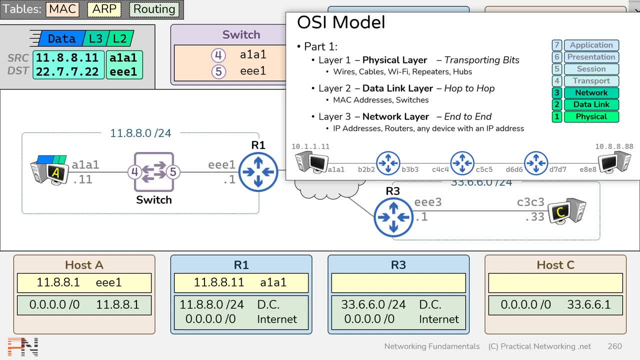 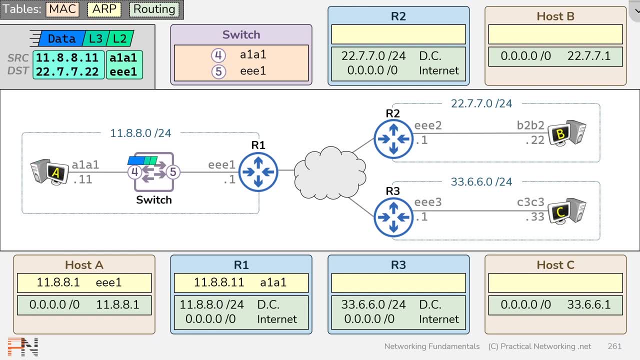 we unpacked it when we discussed the OSI model back in lesson 2.. Either way, host A will put all of this onto the wire, where it'll arrive onto the switch. Once it gets to the switch, the switch will again try and learn what it can from this incoming frame. 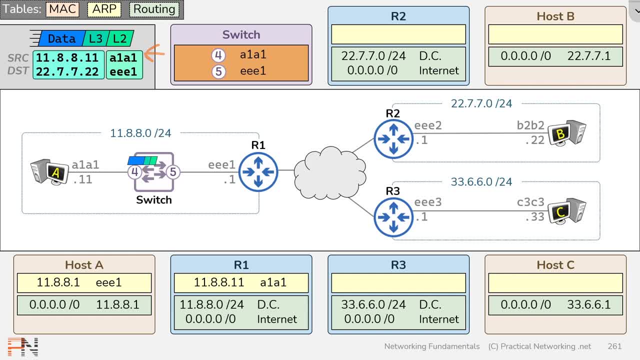 This frame arrived on port 4 and had a source MAC address of A1, A1, and our switch already has that entry in its MAC address table. So there's nothing new for the switch to learn, but this particular entry will be refreshed in the switch's. 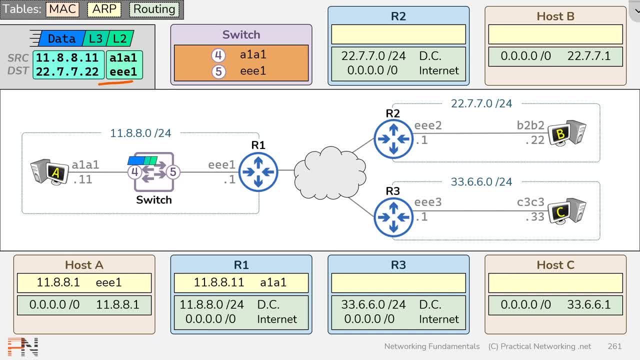 MAC address table. Then again, the switch is going to look at the destination MAC address to determine that this frame should be forwarded out port 5, where it'll put it on the wire and send it out towards router 1.. Once that arrives to router 1, router 1 will strip the Layer 2 header. 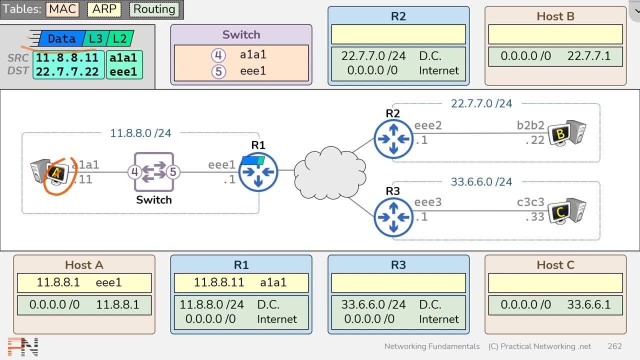 The purpose of that header was again to take the packet from host A to router 1.. It did that successfully and we no longer need it. Then router 1 will take a look at its routing table to determine where it's going to send this packet next. 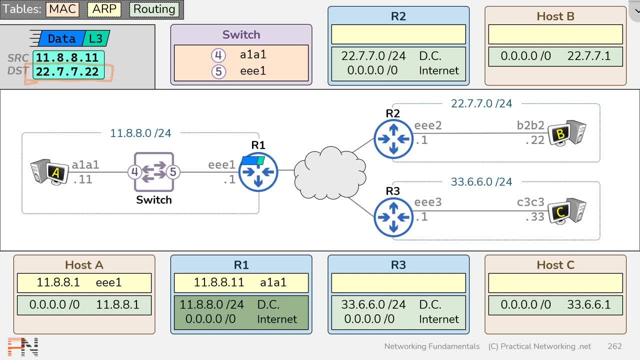 The destination IP address of this packet is the IP address 22.7.7.22,, which matches this route for router 1, which means router 1 knows that this packet is going to be sent across the internet, As we discussed earlier in this module. 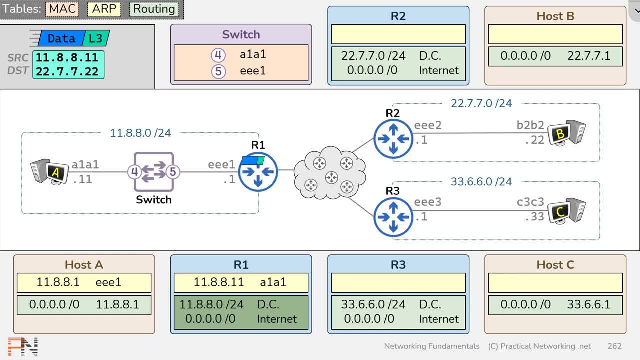 the internet is really just a bunch of other routers that'll hand data off to one another, And normally this route would point specifically to one of these routers, But we unpacked the details of how routers hand data to other routers back in lesson 5,. 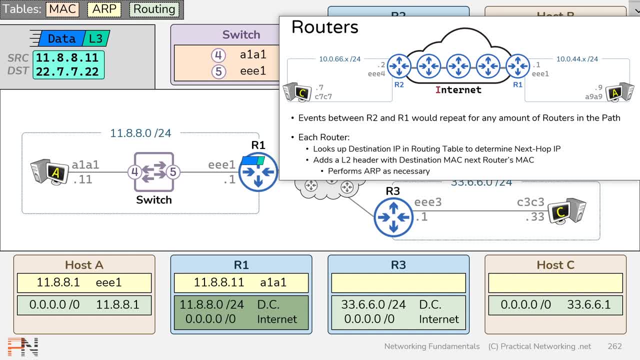 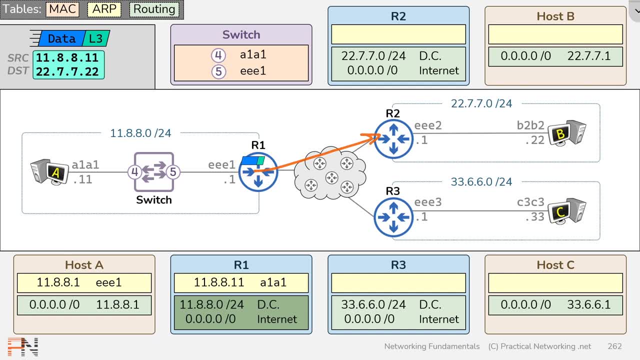 so, rather than repeat myself, I'll simply direct you to that video if you want more information on this process. I'll also mention that there are actually many more ways that this packet can get through the internet to router 2.. These are contained in what's known as WAN technologies. 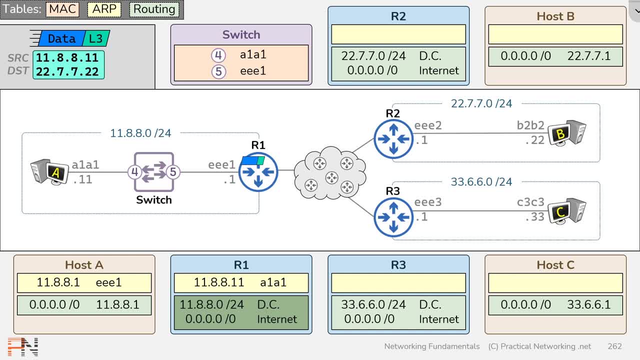 and the details of each of them are outside the scope of this module. One way or another, this packet will be passed from router to router across the internet until it finally gets to router 2.. And when it gets to router 2, router 2 is going to. 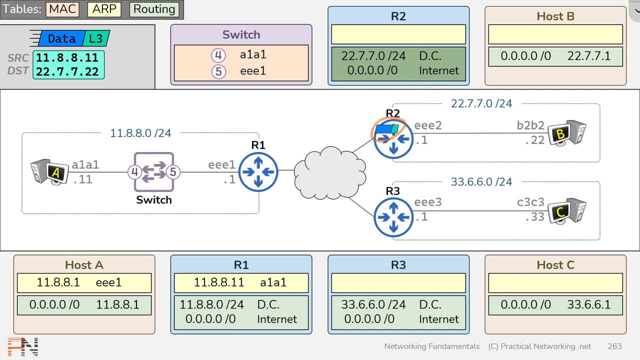 take a look at its routing table to try and figure out how to deliver this packet. The destination IP address of this packet hasn't changed, which means this packet matches this route and router 2 knows it's going to be delivering this packet to its final hop. 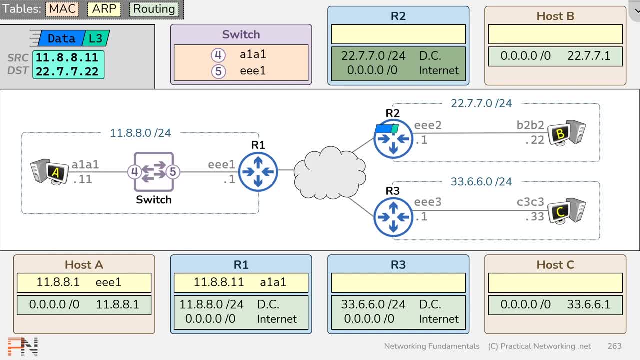 within the directly connected network that router 2 is attached to. However, at this point router 2's ARP table is empty, which means router 2 is unable to put together the layer 2 header necessary to take this packet to host B. So, just like before, 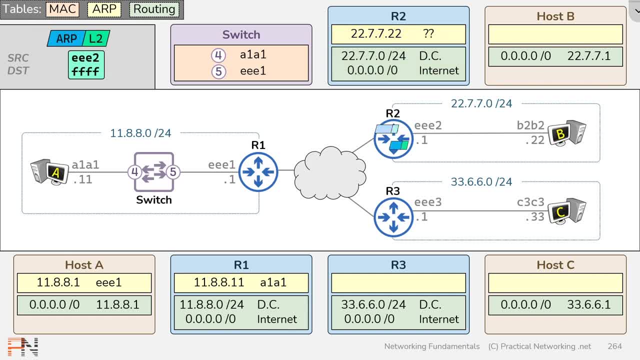 router 2 is going to have to put that packet on hold and send out an ARP request. The ARP request will be sent to the broadcast MAC address, but this time the source MAC address is going to be router 2's MAC address. 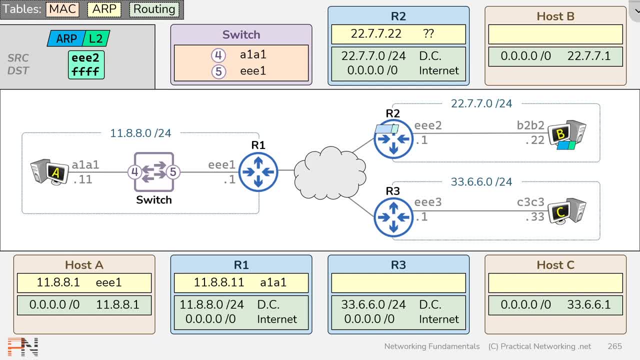 put onto the wire where it'll arrive on host B. Upon receiving the ARP request, host B gets to learn the ARP mapping of the sender of that ARP request. In this case the IP address 22.7.7.1 maps to the MAC address EEE2.. Then host B will generate a response. That ARP response will look. 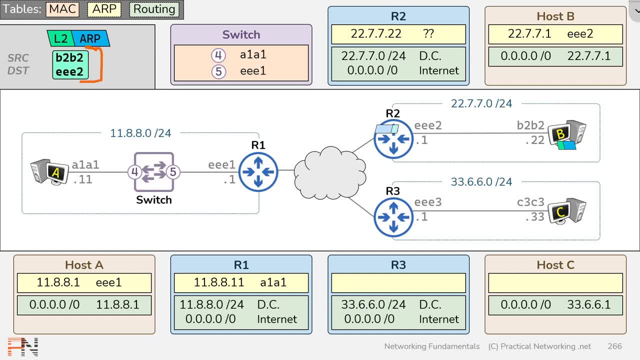 like this: It's going to be a unicast frame sent with a source MAC address of B2B2 and a destination MAC address of EEE2.. That ARP response will be put onto the wire where it'll arrive, on router 2, and router 2 will learn the ARP mapping that it was trying to learn. 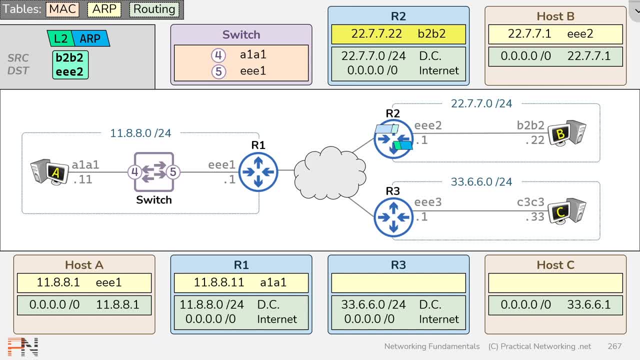 that the IP address 22.7.7.22 maps to the MAC address B2B2.. And now router 2 has all the information necessary to put together the layer 2 header that'll take this packet to host B. That layer 2 header is going to have a source MAC address of router 2. 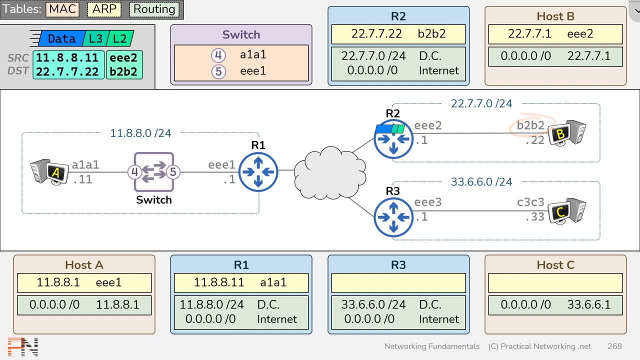 and a destination MAC address of host B Router 2 can now put the packet on the wire where it'll finally arrive on host B. Now, normally you wouldn't see a host plugged directly into a router. Normally this host would be connected to a switch, which would then possibly be connected to other 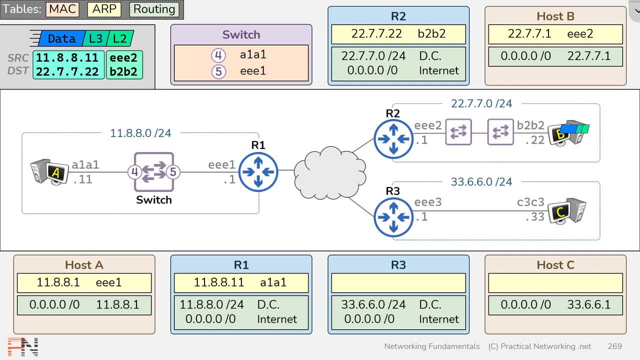 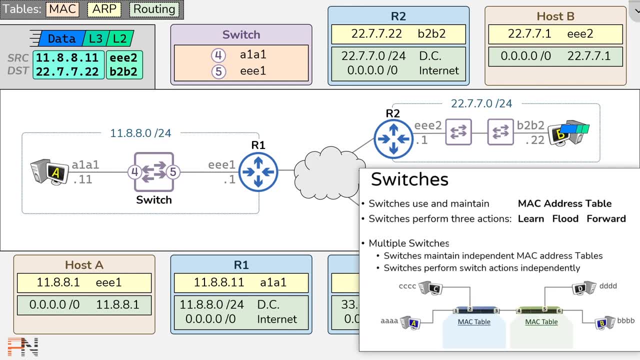 switches which would then finally connect to the router. But we've already illustrated a switch's operation back here and we discussed how frames travel through multiple switches back in lesson 4.. Keep things simple: this network does not have any switches, But if you want to understand how data 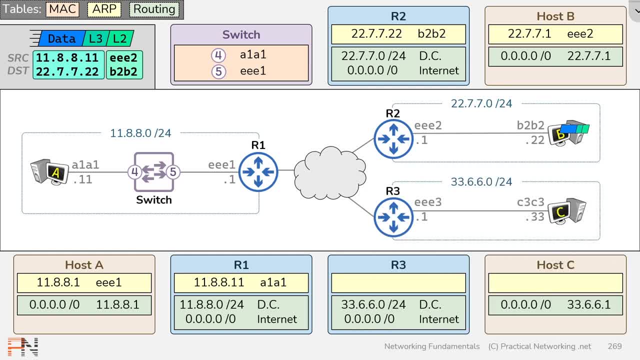 flows through multiple switches. check out lesson 4.. Either way, once this packet arrives on host B, the first thing host B does is strip the layer 2 header Again. that header only existed to take this packet from router 2 to host B. The next thing host B does is strip the layer 3 header. 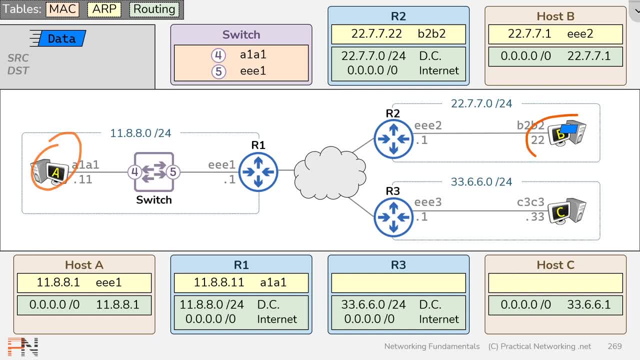 Again, the purpose of that header was to handle the end-to-end delivery of this data, Which it did so successfully, And now host B can finally process all those 1s and 0s contained within that data payload. Once it's processed that data, it can now generate a response, And that response. 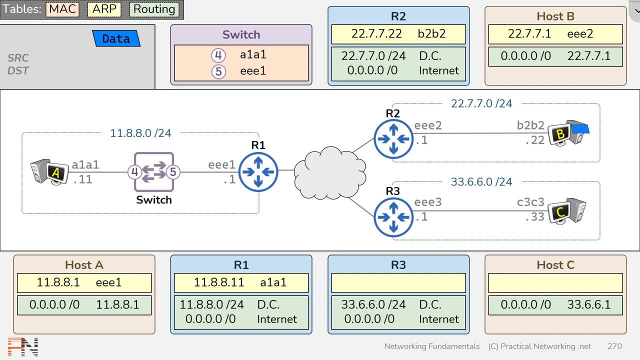 just like before, is simply a data payload which includes a bunch of 1s and 0s, And now we'll step through all the steps required to get this data payload back through the network to host A. What you'll see is that this is going to go much quicker than before. 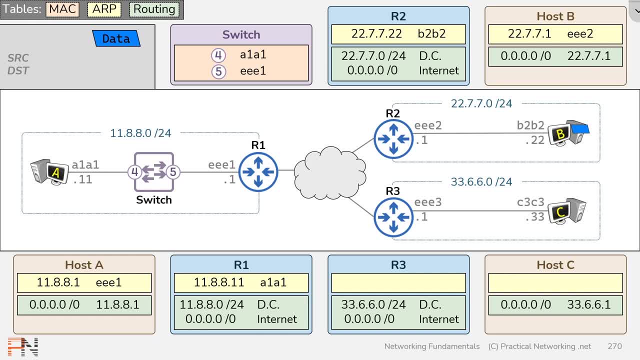 Because this is going to go much faster than before. Because this is going to go much faster than before, Most of our tables have already been populated. Host B will start by throwing a layer 3 header onto that data. That layer 3 header is going to have a source IP address of host B and a destination. 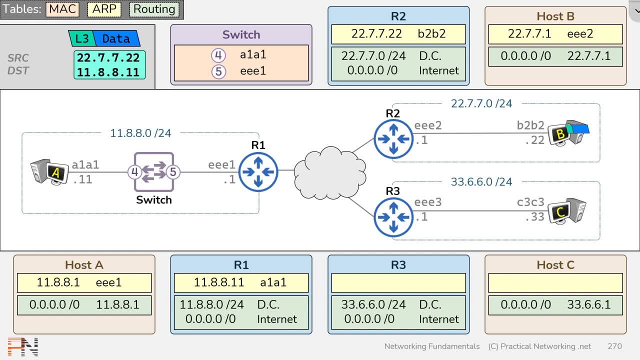 IP address of host A. In this case, since this packet is going to something on a foreign network, we know that it must be sent to router 2's IP address, And at this point host B already has the ARP mapping for router 2's IP address and can therefore already put together the layer 2 header. 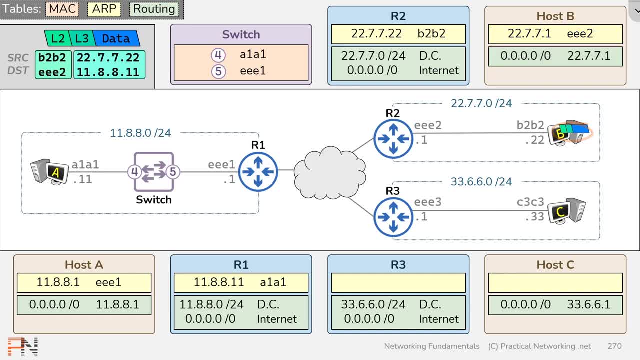 necessary to get this packet across its first hop. This is what will allow this packet to make it across this hop. Upon arriving on router 2,, router 2 will strip the layer 2 header, And then router 2 will take a look at its routing table to figure out where this packet should go next. In this case, 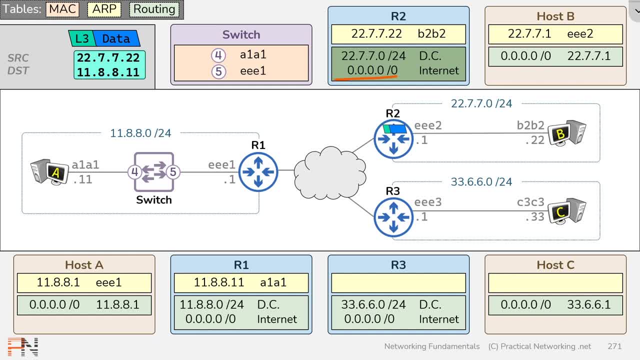 the destination IP address 11.8.8.11, only matches the default route. So router 2 knows that this is going to be sent out towards the internet And again we've abstracted that process out, so it will be handed out from router to router across the internet. 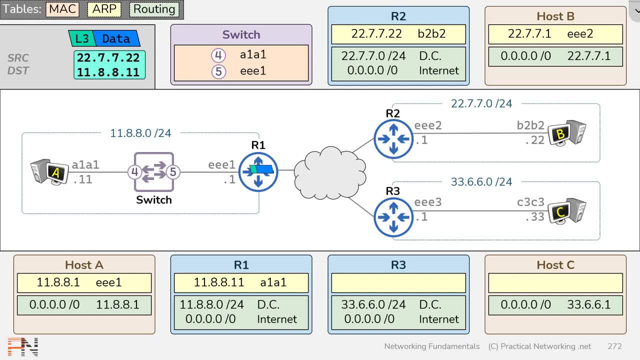 where it will finally arrive on router 1.. Upon arriving on router 1, router 1 will take a look at its routing table to determine that the destination IP address matches the directly connected route. So router 1 knows that this destination IP address is the final hop for. 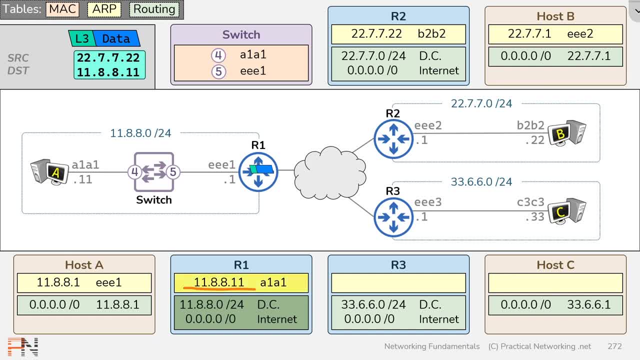 this particular packet And router 1 also happens to already know the MAC address for that particular IP address. So router 1 has all the necessary information to put the packet into this packet. a layer 2 header that'll take this packet across its final hop. That layer 2 header is going to. 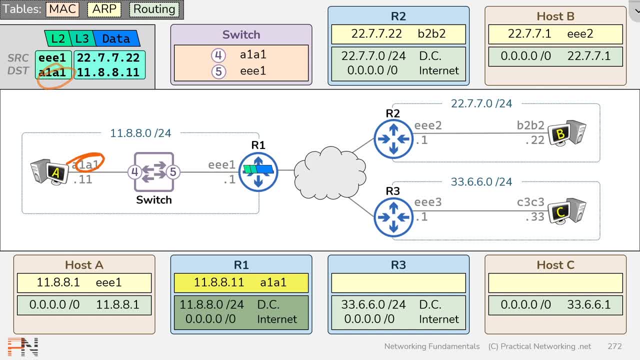 have a source MAC address of router 1 and a destination MAC address of host. A Router 1 can then put that packet onto the wire. It'll arrive on our switch and, just like before our switch is going to try to learn, It'll try and map the receiving switch port, which is 5, to the source. 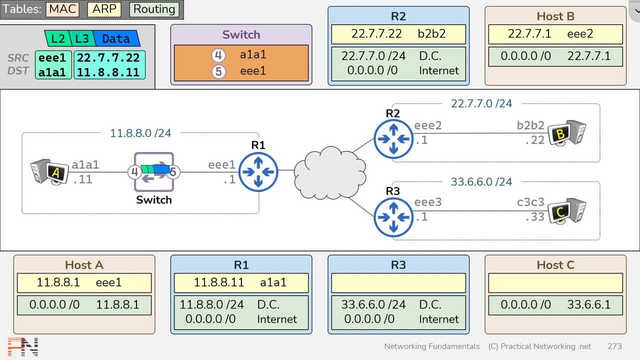 MAC address of the incoming frame, EEE1, and it'll notice that it already has that entry in its MAC address table. So there's nothing new to learn. So this entry will simply be refreshed in the switch's MAC address table. Then the switch will look at the destination MAC address, A1A1, and the 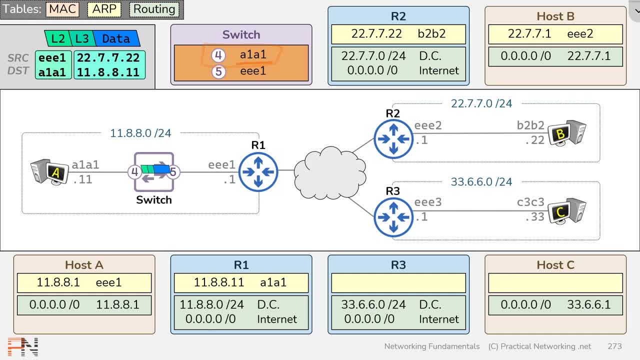 switch knows how to deliver a frame to the destination MAC address A1A1.. This frame will be sent out port 4.. It'll then finally arrive back on host A. Host A will strip the layer 2 header Again. that header took the packet from this NIC to this NIC. Host A will then strip the layer. 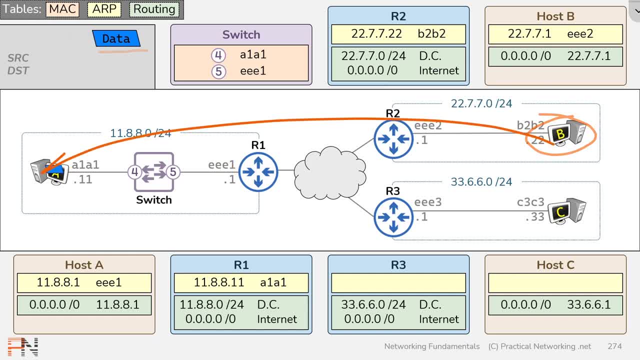 2 header. Host A will then strip the layer 2 header. Host A will then strip the layer 2 header 3 header, which took the data from this end to this end, and finally host A will process that response data. So we just showed you everything that happens to get data from host A all the way. 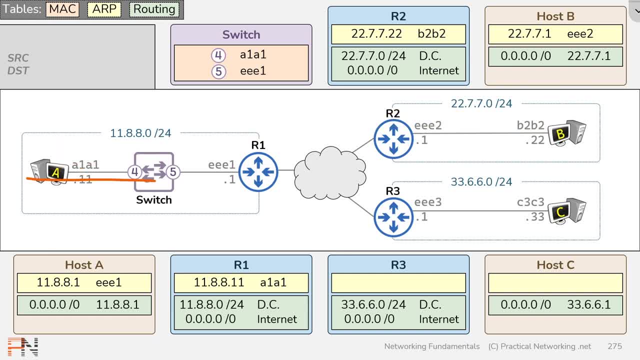 to host B and back again, And we showed you how each of the devices involved in this process used a MAC address table, an ARP table and a routing table to make that happen. Next, host A is going to send some data to host C. Now, if you feel that this has, 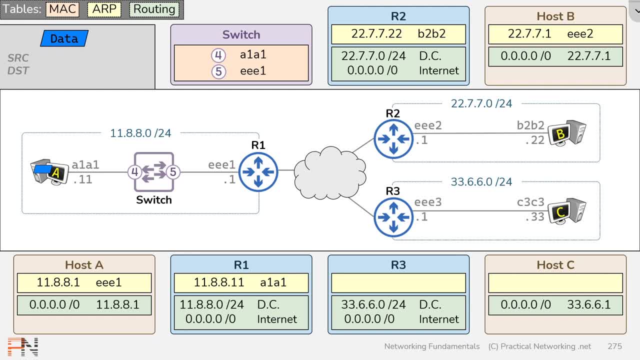 beginning to get repetitive. awesome, That's great, That's exactly right, and it means you're learning how it all works. Remember: all these devices- host switches, routers- all follow simple, consistent packet processing rules. If you understand those rules, you can scale this. 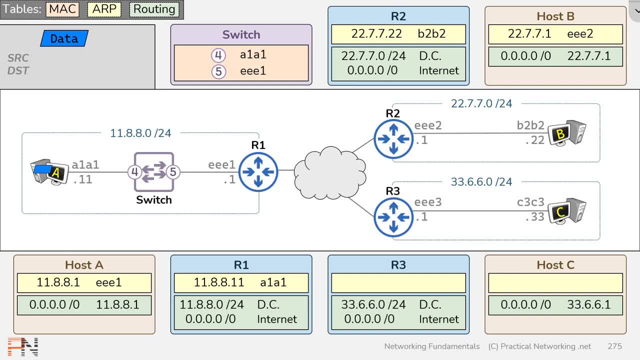 topology to hundreds of devices and still walk your way through each step necessary For this last packet, going from host A to host C. I want you to test yourself. Try to guess what happens next at each step just before I explain, With that in mind, the first thing that host A does to send this data to host C. 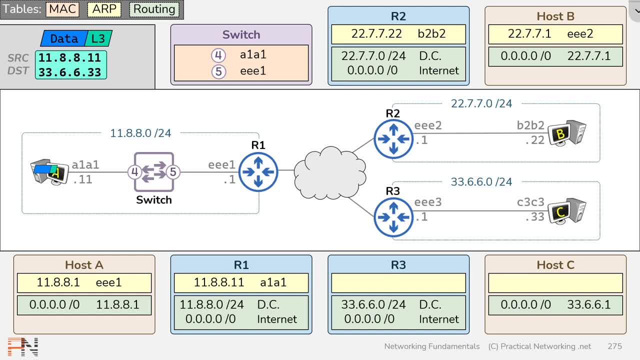 is throw a layer 3 header onto that data. That layer 3 header is going to have a source IP address of host A and a destination IP address of host C. Then, since host A knows this packet is going to a foreign network, host A is going to look at its default route to determine the default. 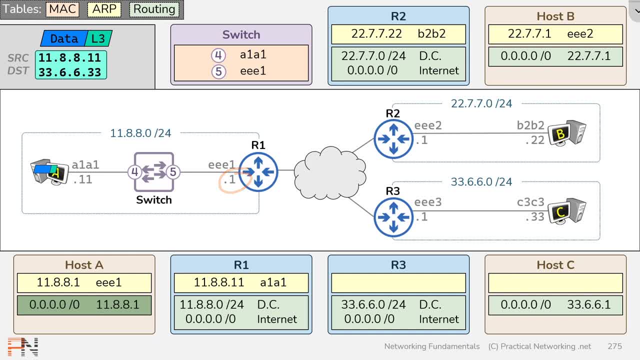 gateway's IP address, which is router 1.. And since host A already has the ARP mapping for its default gateway's IP address, you can already put together the layer 2 header which will take the packet to router 1.. That layer 2 header will have a source MAC address of host A and a destination. 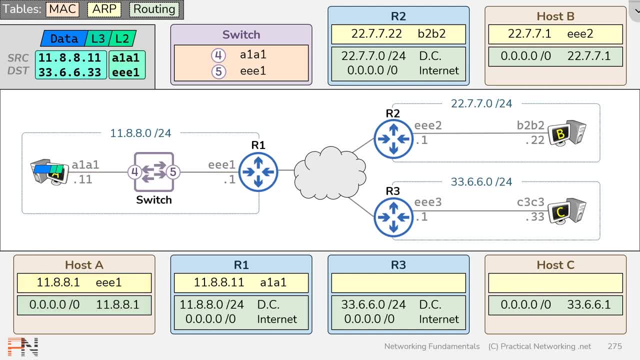 MAC address of router 1.. Host A will put this onto the wire where it'll arrive on the switch. The switch will try and update its MAC address table with an entry for port 4, mapping to the source MC address A1- A1.. Since that entry already exists, that entry is simply: 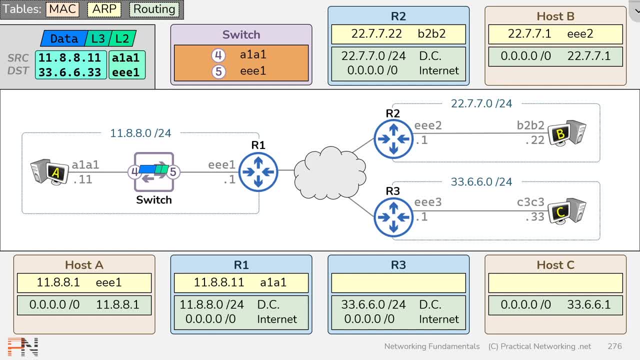 going to be refreshed in the MAC address table That Move DéPljd is simply going to multiply the is going to look at the destination MAC address to determine where to send this packet next. That MAC address exists out port 5, which will have this switch. send this frame out port 5.. 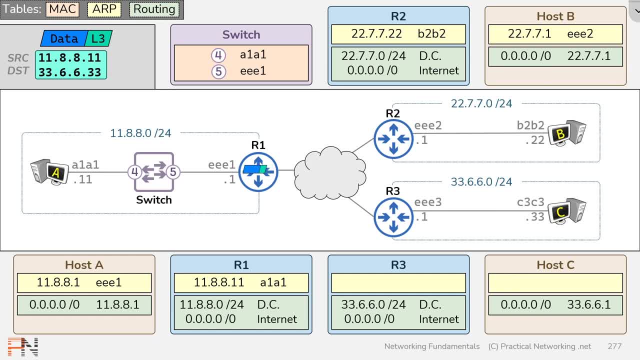 It'll then arrive on the router and the router is going to strip the layer 2 header. and now router 1 is going to look at its routing table to determine where to send this packet next. The destination IP address on this packet matches the default route, which means router 1 is going. 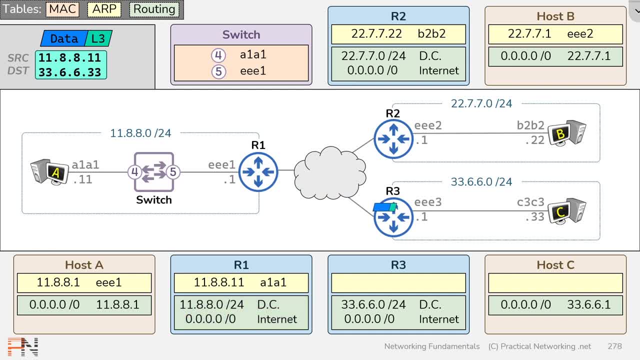 to send this packet across the internet where it'll finally arrive on router 3.. When router 3 gets it, router 3 is going to again look at the destination IP address and determine that it matches the directly connected route in router 3's routing table. This tells router 3 that it's going. 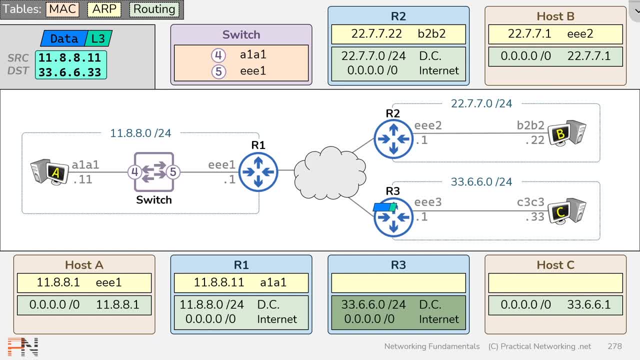 to have to put a layer 2 header onto this packet that matches the MAC address associated with this IP address, right here. But at this point router 3 does not have anything in its ARP table, so it cannot put together the appropriate routing table. Therefore, just like before, router 3 is going to put that packet on hold and then router 3 is going. 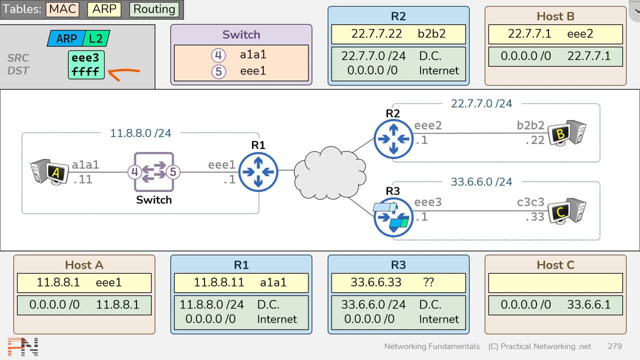 to send out an ARP request. That ARP request will be sent to the broadcast MAC address, which will ensure that this ARP request gets delivered to everybody on this particular network, Which means host c will definitely receive that ARP request. Upon receiving the ARP request, host. 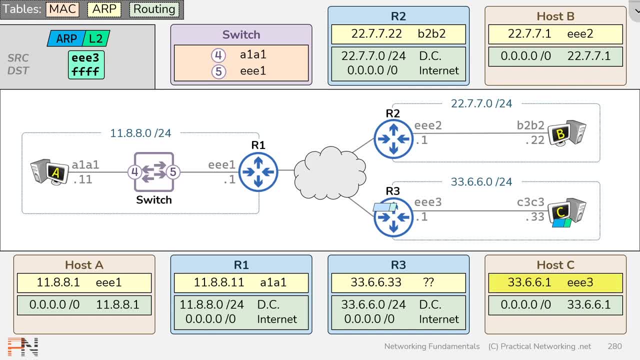 c will learn the ARP mapping of the sender of that ARP request, which in this case is the IP address 33.6.6.1 and the MAC address eee3.. Then host c will put together the ARP response. That ARP response will look like this: The ARP response is sent as a unicast frame. 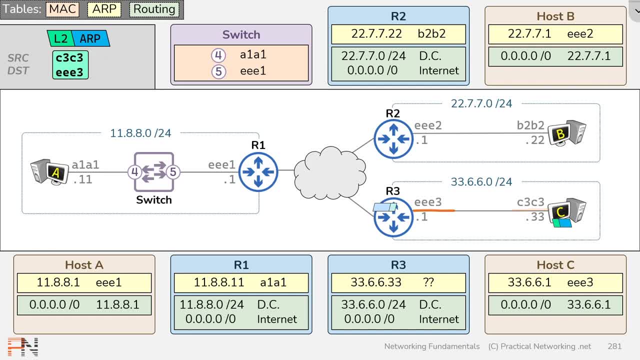 meaning it's going from a specific MAC address to another specific MAC address. This will get the ARP response back to router 3 and then router 3 will finally learn the ARP mapping it was trying to learn, And now router 3 has everything it needs to put together the 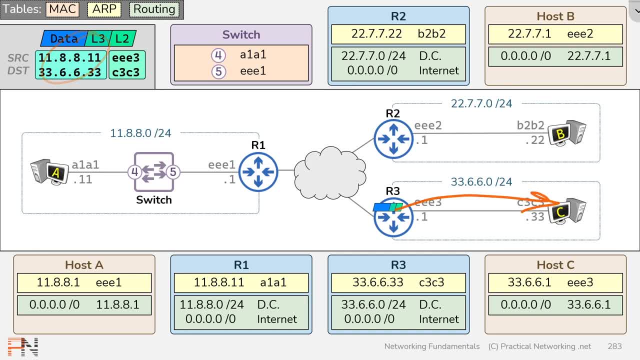 array of commands to set up the ARP response By simply Pence toхop andget the ARP response. it also storesosing theroffenance id. The router 3 will now be able to send работrage input in a frozen shell set that can be moved to another anchor host or to create a new router. 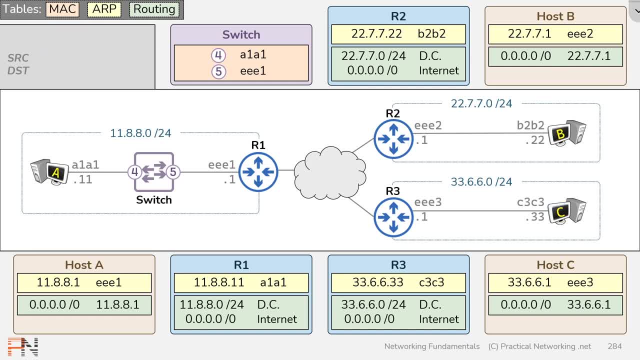 So once the clean hangoutIt format alights our WomenSouve Router, we will no longer get alive. MotoVersion of an ARP file in our manager core server版dot connector. All of these commands that has been set up are going to remain in print. 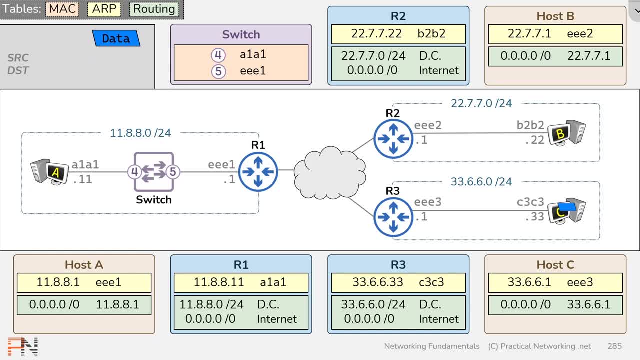 So now host c is going to destroy all his ARP response calls and continue on higher и低 and higher and a higher e onto that packet. That layer three header is going to have a source IP address of host C and a destination IP address of host A. Host C knows it's trying to speak to something on a. 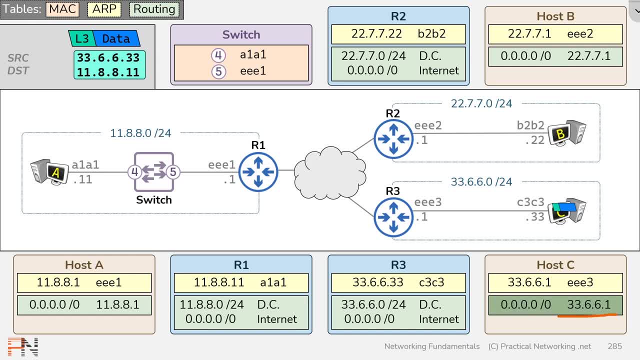 network. So host C knows that this must be sent to the default gateway, In this case router three. And host C happens to already have the ARP mapping for the default gateway, So it has all the information it needs to put together this layer two header which includes the destination MAC. 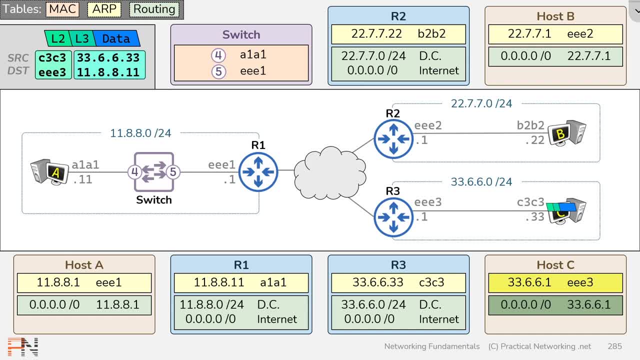 address of router three, Host C, will put that onto the wire where it'll arrive on router three. Router three will strip the layer two header And then router three will take a look at its routing table to determine where to send this packet. The destination IP address of this packet: 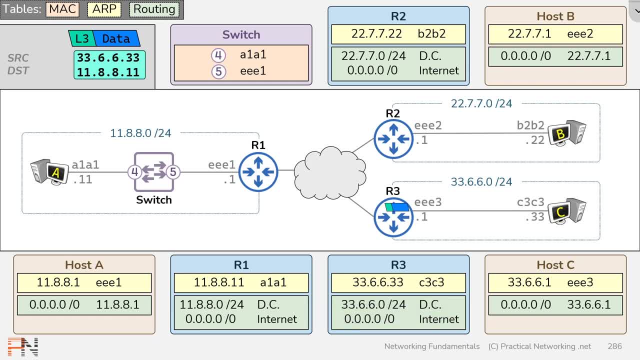 matches the default route. So router three will send that packet out towards the internet, where it'll finally arrive on router one. Router one will take a look at its routing table and compare the destination IP address to see if it's sent to the default gateway. 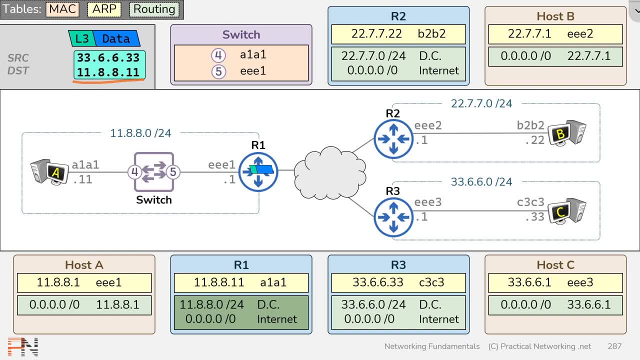 Which route matches. In this case, this destination IP address matches our directly connected route, which means router. one knows that this packet will be delivered to its final hop And router. one happens to already know the ARP mapping for this particular destination IP address. 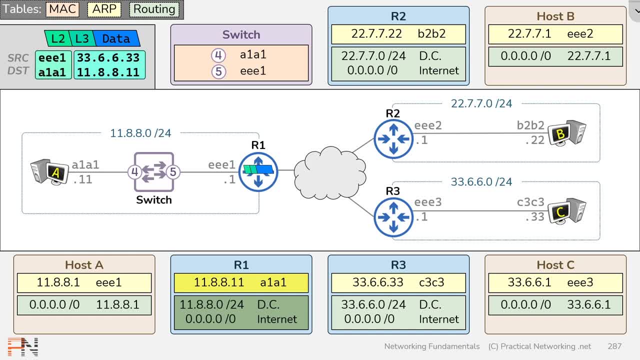 So router one has all the necessary information to put together a layer two header with a source MAC address of router one and a destination MAC address of host A. That will get sent onto the wire where it'll arrive on the switch, And host C will send that packet out towards the internet. 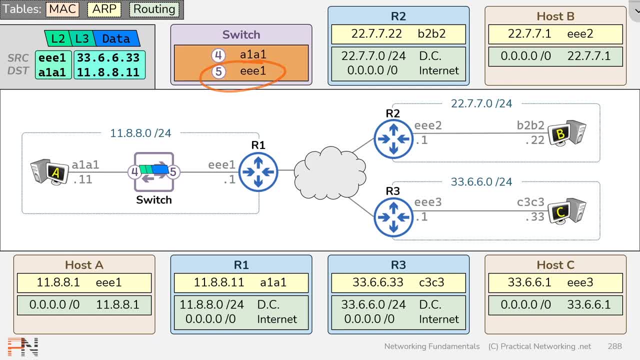 and again, the switch has nothing new to learn, So it'll simply refresh that entry in its MAC address table. Then the switch will look at the destination MAC address to determine that this frame should be sent out port four. The switch will put that onto the wire where it'll arrive. 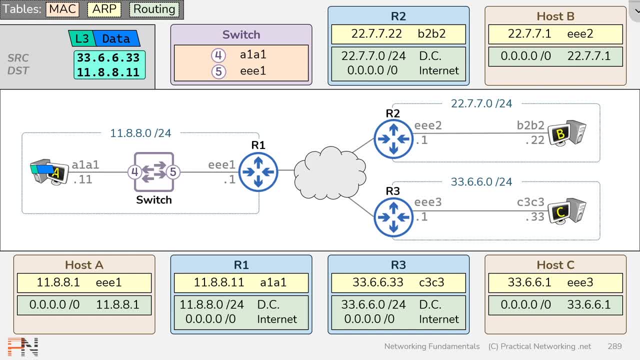 on host A. Host A will then strip the layer two header. Host A will then strip the layer three header And, finally, host A will process the response from host C. And that, my friends, is every single thing you need to know about router three. So let's get started. 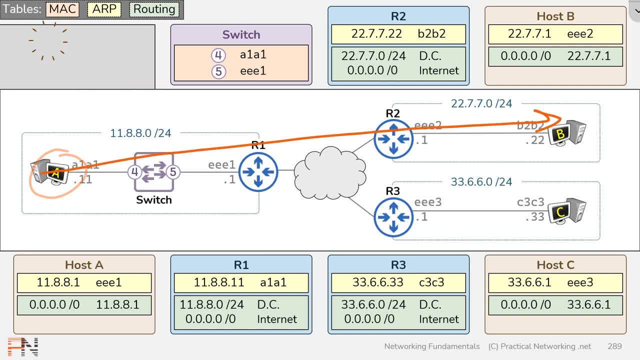 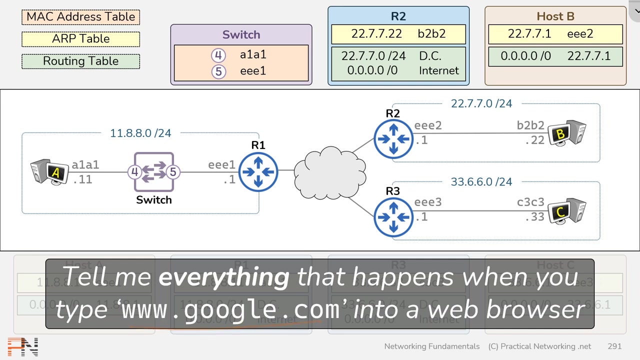 The last idea I want to leave you with has to do with a very common interview questions for networking engineering type roles. That interview question looks something like this: Tell me everything that happens when you type wwwgooglecom. This question is trying to see if you can apply what we learned in this video to the simple act. 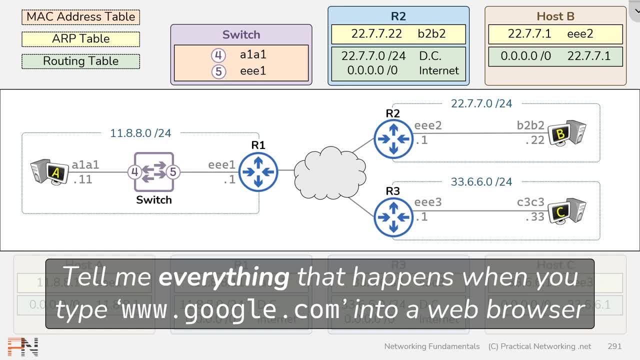 of visiting a website. Browsing to a website essentially involves two phases: First, using DNS to resolve a domain name into an IP address And second, sending an HTTP request to that IP address. Well, in our illustration, the first thing we did was send a packet from host A to host B. 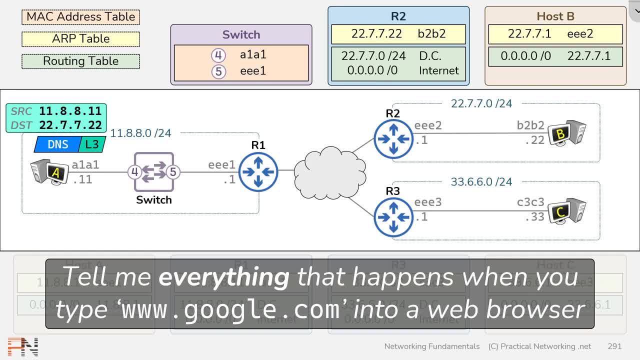 But what if this packet was sent from host A to host B? Well, in our illustration, the first thing we did was send a packet from host A to host B. But what if this packet was actually a DNS request? And what if host B was actually a DNS server? The response from the DNS server would have given us. 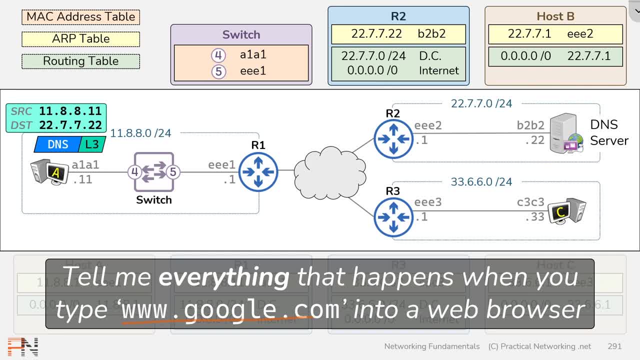 the IP address of the web server for the domain you're trying to visit. What if that web server was actually host C? Then that packet that we sent from host A to host C would have actually been an HTTP request. So you see, everything we did in this video was in service of answering this. 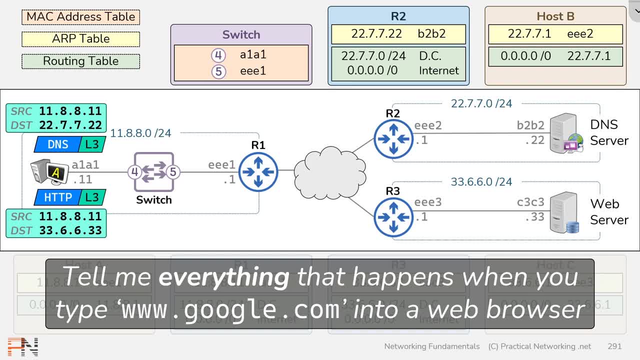 very common interview question, And now you can confidently answer this question when you inevitably come across it. But it's more than just an interview question, though. It's a fundamental part of understanding how internet connectivity works Next time your friend or coworker or